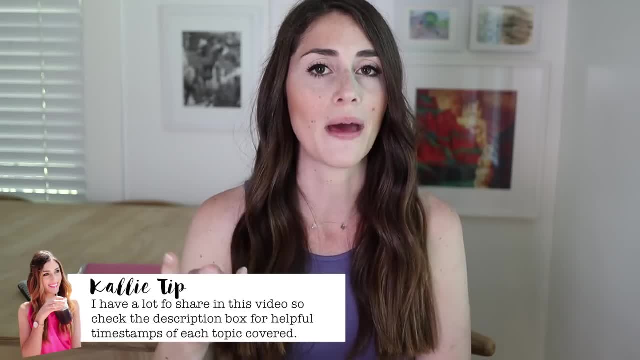 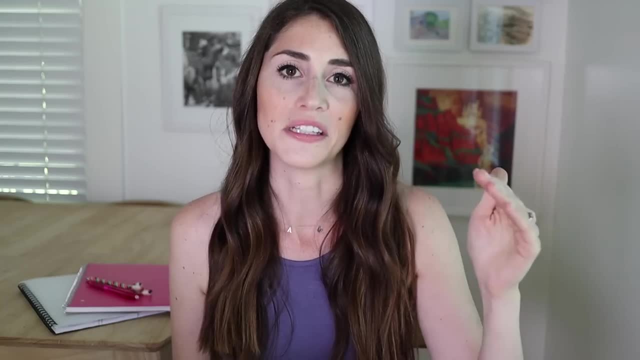 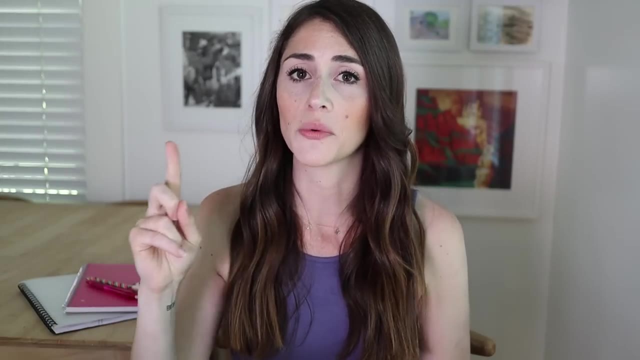 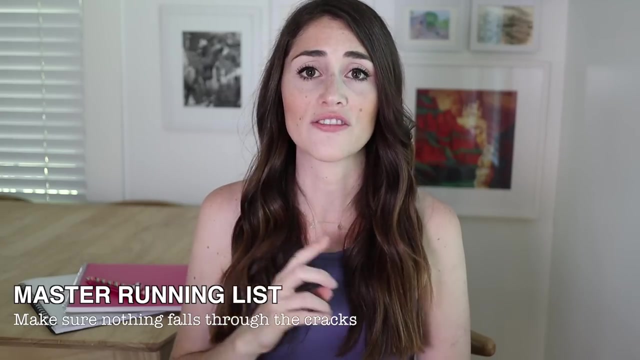 And so what I want to do is I want to break down essentially the two main methods that I use for planning and scheduling that have allowed me to get back to a level of productivity that I feel really happy about. So, in general, I use two basic methods to get stuff done. The first one is what I call the master running list, And what this does is it allows me to make sure that nothing is falling through the cracks, nothing gets forgotten. 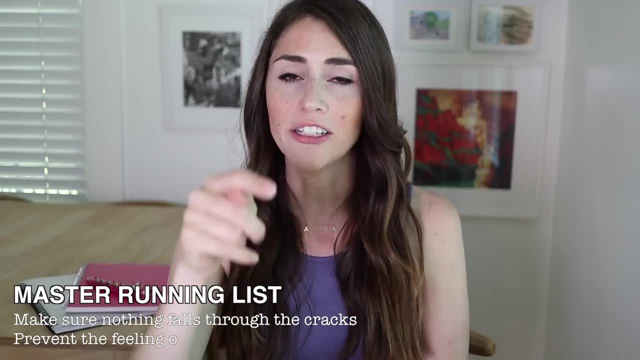 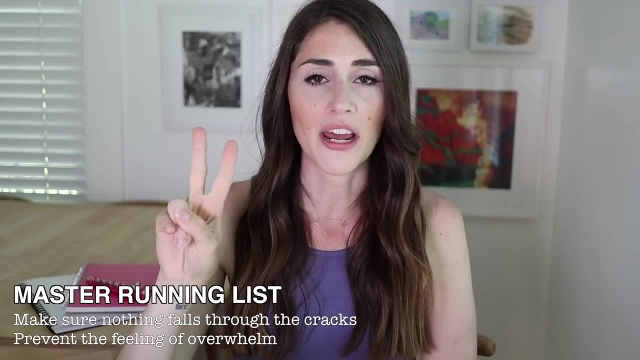 But, more importantly, it's what helps me tackle that feeling of overwhelm, Like I have so much to do and I have no idea how I'm ever going to get it done. And then the second method that I use in conjunction with that is time blocking. 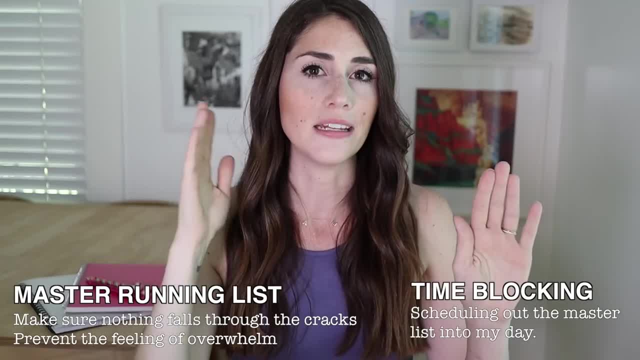 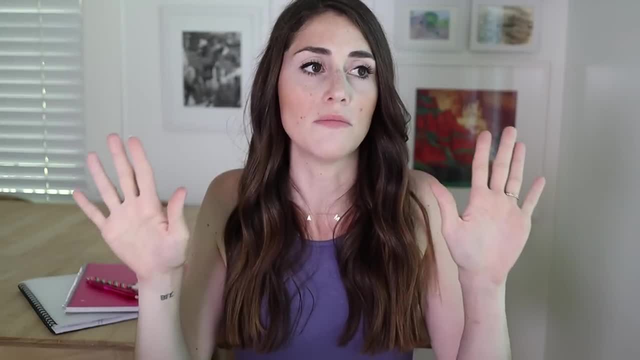 And time blocking is how I take that list and I actually block it into times of space so that I can get it done. And the beautiful thing about this method is you don't have to be some sort of organizing genius. Everything that I use for all of my scheduling lives right inside of these two notebooks. 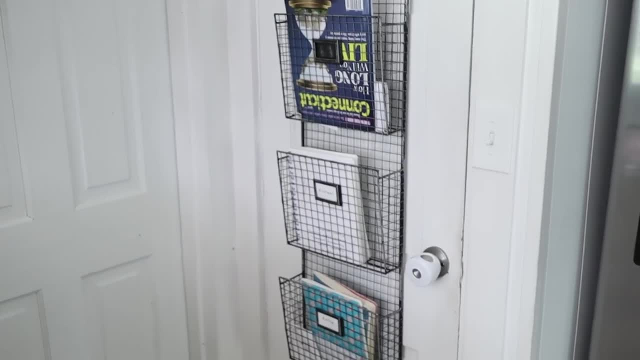 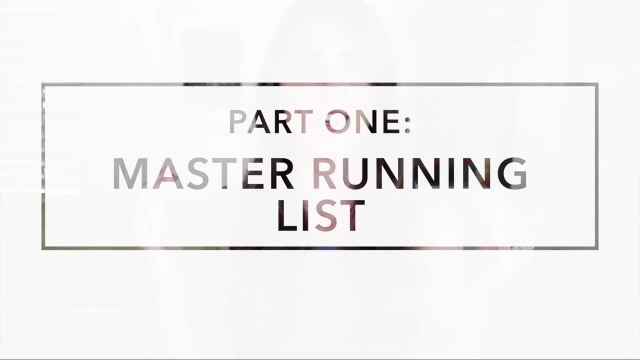 And then they just hang right in my kitchen on a paper organizer that I have And I just put it right in there. It's very minimal, it's not complicated, it's easy, it's portable. So method one of two for my scheduling and productivity is the master running list. 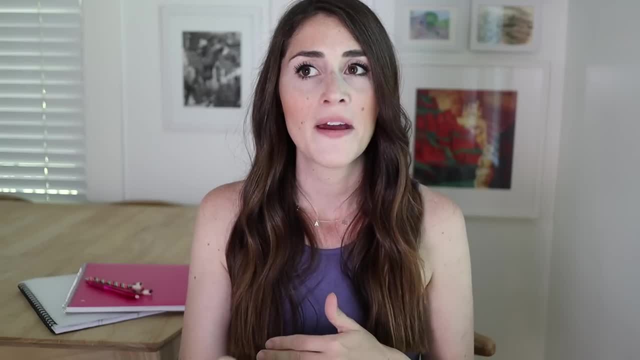 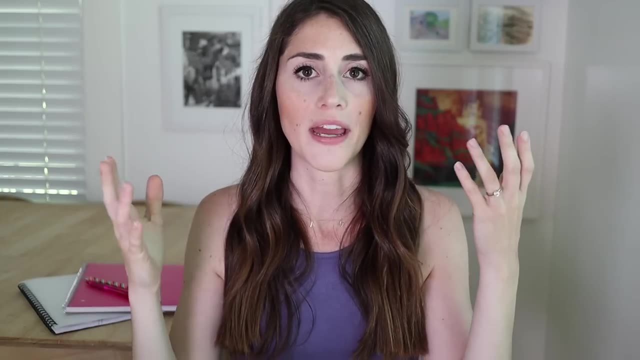 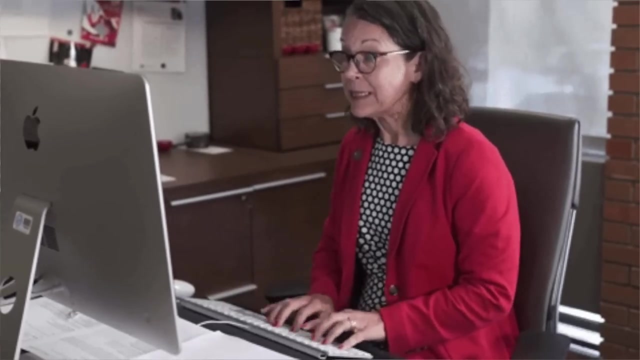 And this is something that I've sort of had to invent into my life because I very much struggled with the issue of overwhelm. I just would have 800 tabs open in my brain of 800 different things that I wanted to do And I would constantly feel overwhelmed of how was I ever going to get it done? where was I supposed to start? 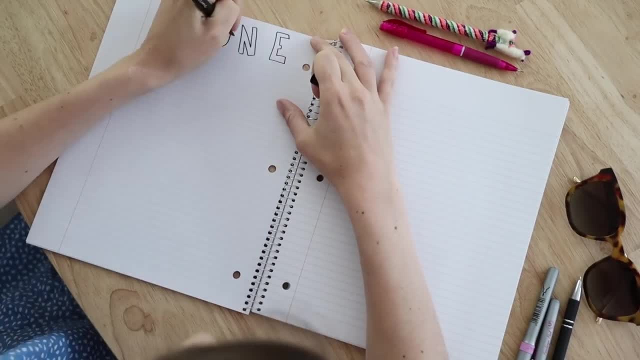 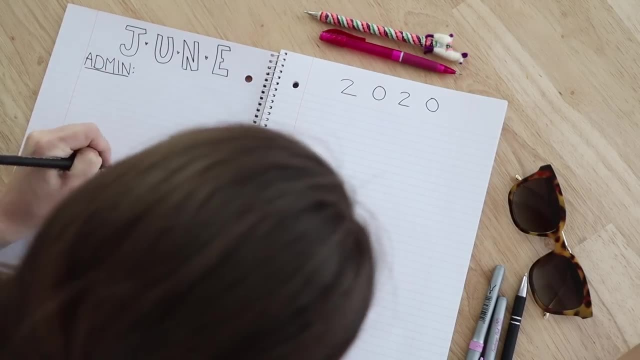 To solve this problem, I adopted my running master list. Now, these don't need to be anything fancy or pretty. Mine are jotted down in a one dollar notebook And I have a master list for each month, and then that month is broken down into each week. 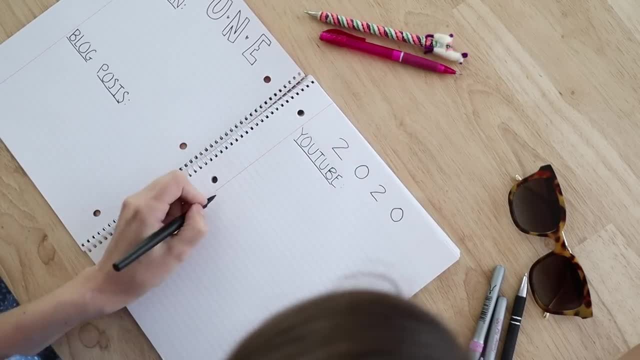 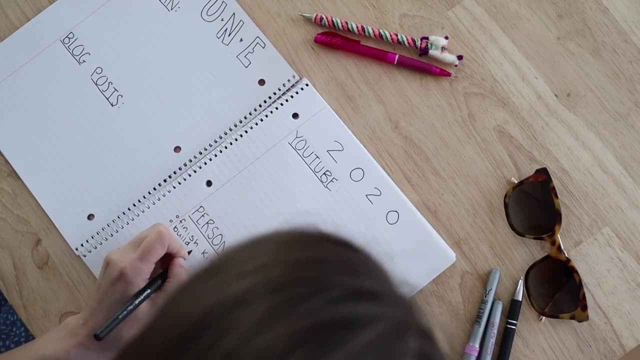 Now, my monthly list is something that I sit down at the very beginning of the month, usually a couple days before the first of the month, And I start to write down all of the things that I want to get accomplished that month. I personally break it into a couple of categories. 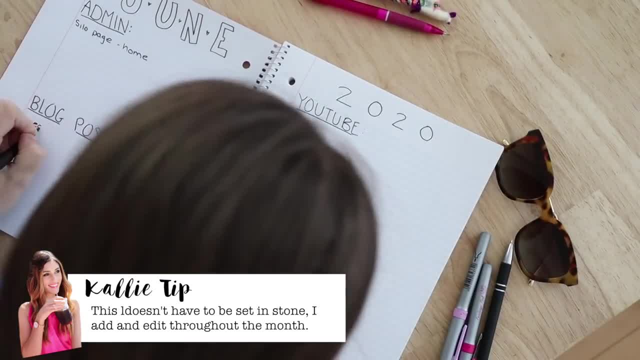 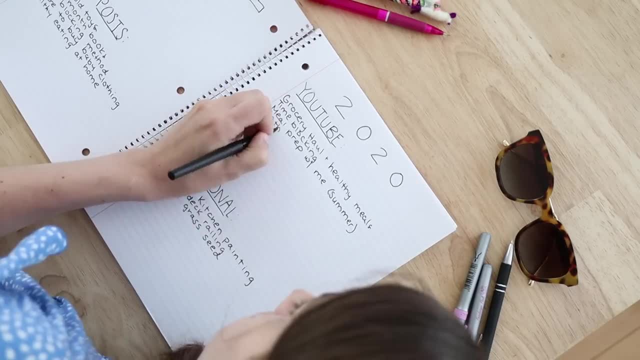 So this is going to vary for each person. For me, I have one that is blog posts, one that's YouTube videos, One that's admin and backend work, and then one that's personal stuff. You're going to use whatever categories work for you. 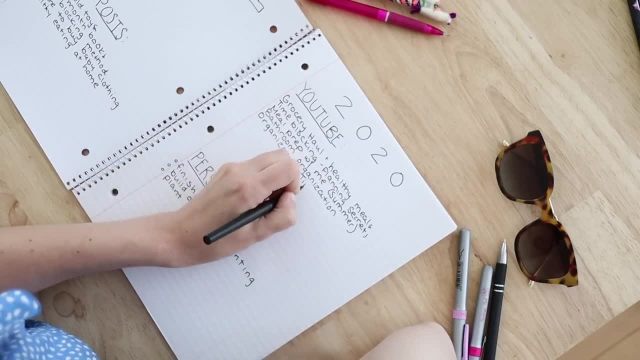 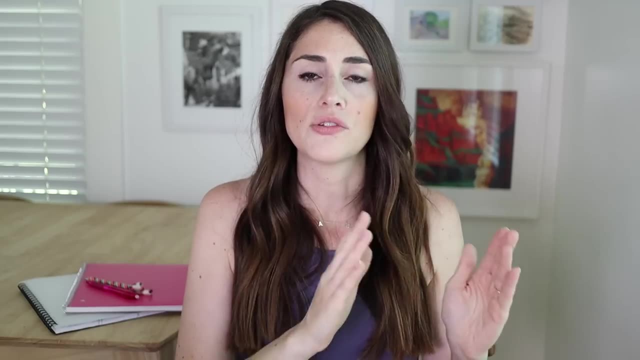 Maybe you're going to have one that's home projects, one that's stuff for kids, one that's work related, one that's personal. You may only have two categories, and that's totally fine, But it allows you to sort of bucket your different hats that you wear. 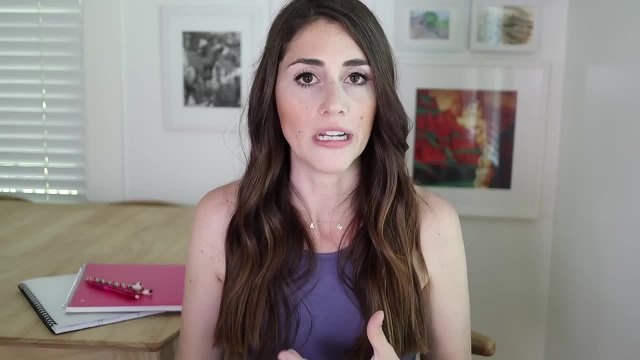 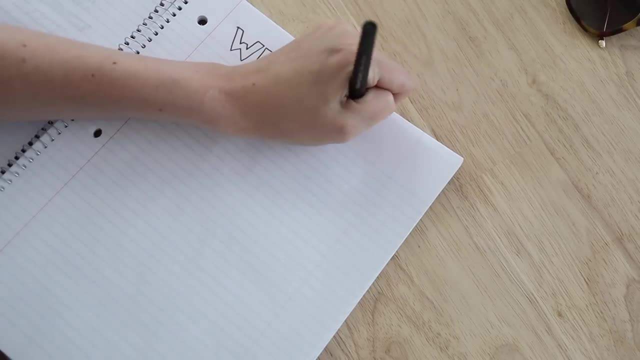 I think a lot of us sometimes feel like we're juggling a lot and we're wearing a lot of hats. So break it down into those different hats that you wear. Then the next thing I have is my weekly list, And this is where I break down the bigger 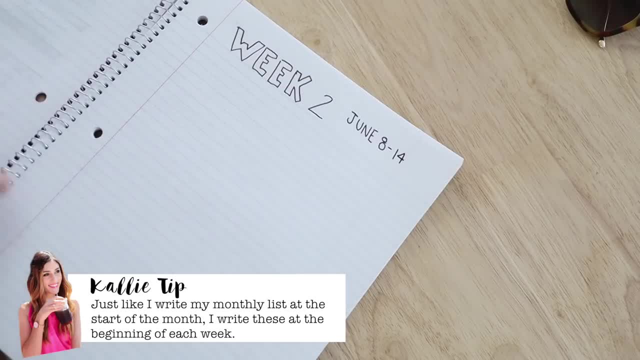 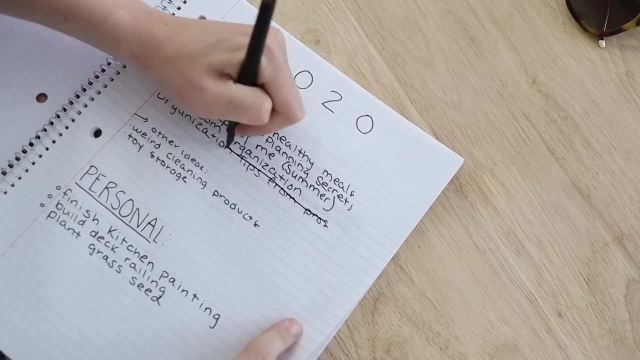 projects into smaller tasks that are needed to complete them. So maybe on a monthly list, one of my big tasks is I have a YouTube video that I'm working on. Some of the smaller tasks that might fit into there would be writing my script. 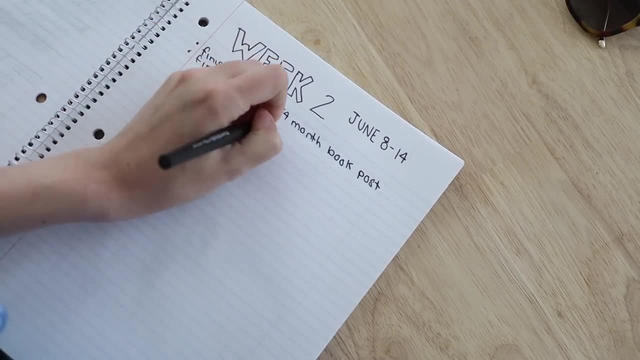 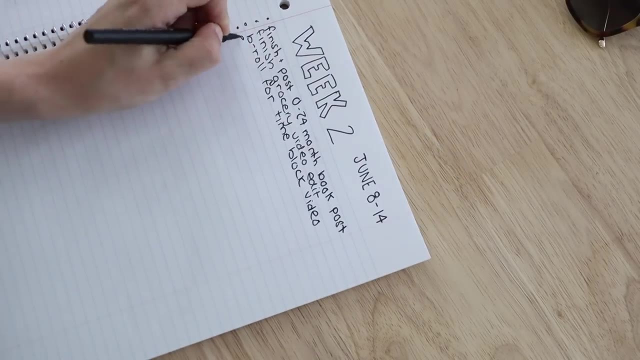 doing research, for you know, whatever I need to do in the video- different shots that I need to get, creating the thumbnail, editing the video- And often I'm not even doing all of these smaller tasks inside of a single week. Maybe I'm doing a couple of tasks for one bigger project and a couple of tasks for another project. 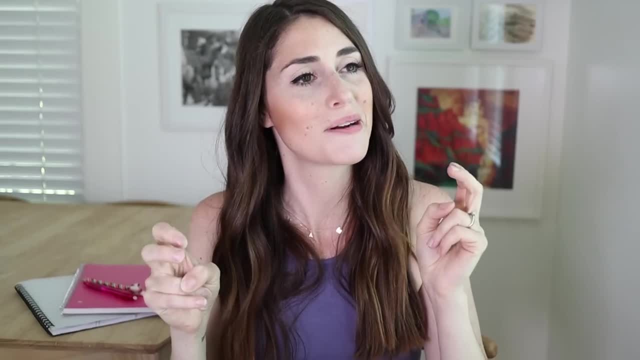 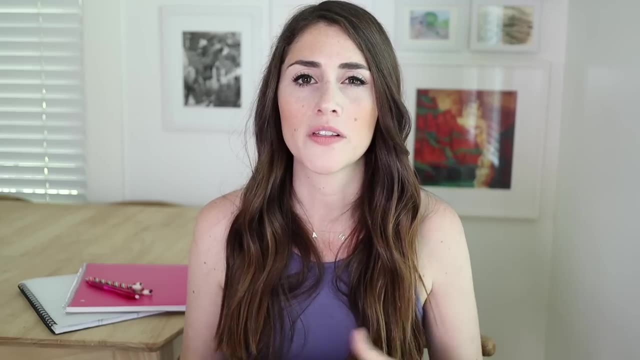 Now the reason that my running master list- what am I calling it Super master running list? Now the reason that my master running list really works is twofold. The first reason that works really well is because it's essentially a brain dump. 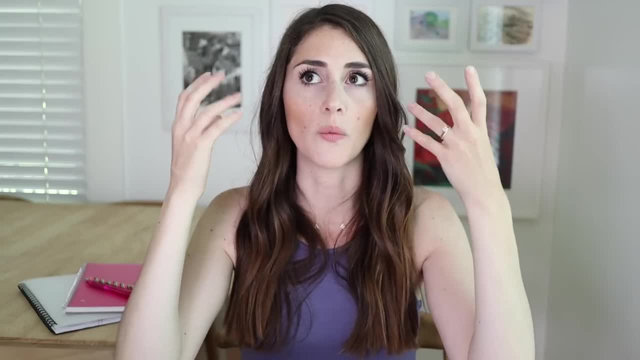 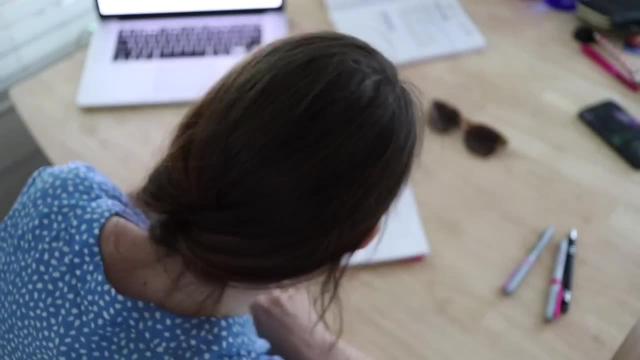 It allows you to put all of the thoughts and all the things that you are feeling overwhelmed about that you need to get done onto a piece of paper, And that can be extremely cathartic. I'm going to share with you, under time blocking, how I actually take this list. 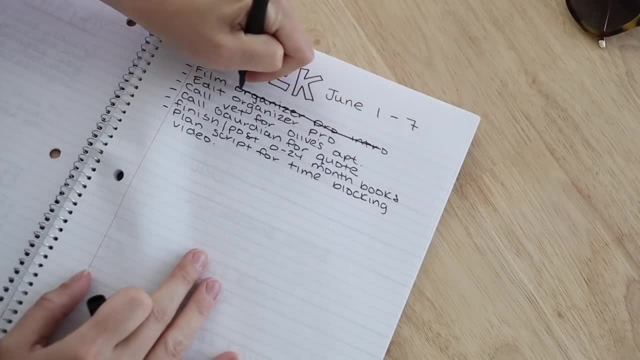 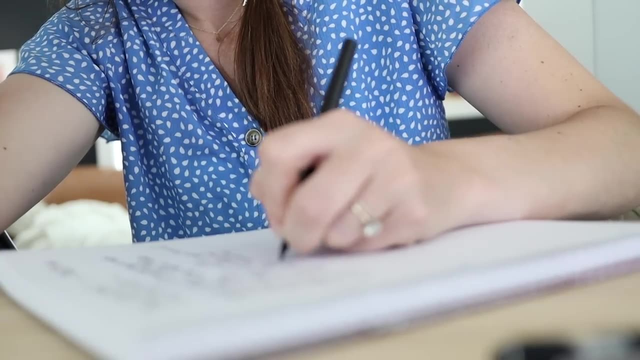 and then work it into getting it done. But this process is about just dumping all of those things that you have in your brain onto a piece of paper. It allows you to close some of those tabs that you have open inside of your brain, And seeing it laid out on a piece of paper is, honestly, the first step. 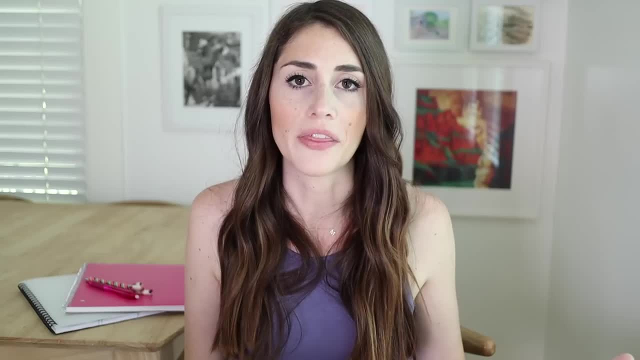 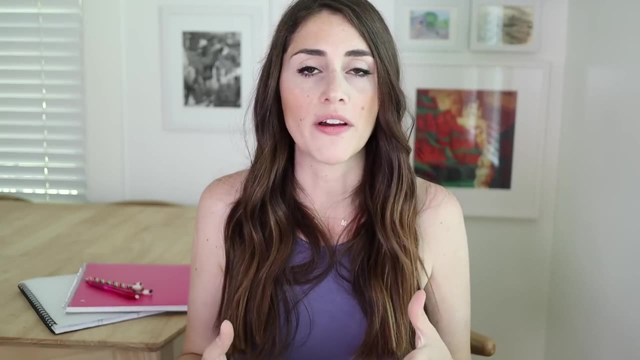 The second reason that I love my running master list is because it allows me to stay accountable for things. It doesn't allow anything to fall through the crack. It doesn't allow anything to get forgotten. We all know that with scheduling, you know we have really great intentions but life happens. 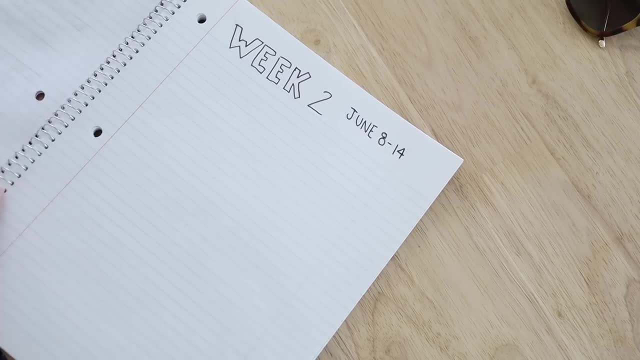 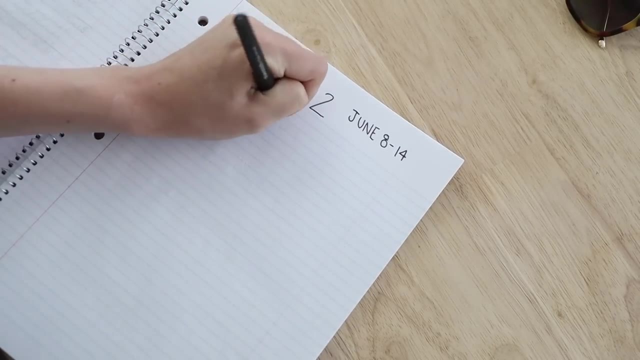 Maybe you had a busier month than you plan to. If something doesn't get done that week or that month, the very first thing I do when I start a new monthly or weekly list is I reference the one before that so that I can bring anything that was not completed over to this week. 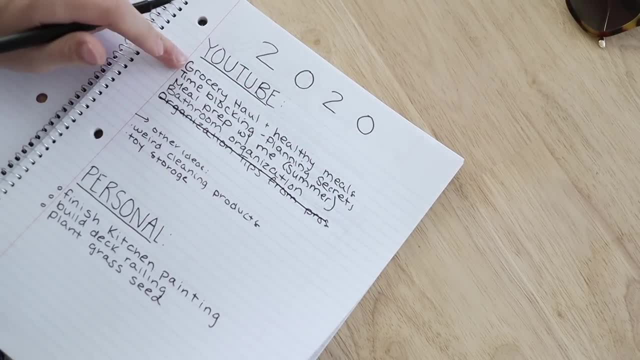 So maybe you had a list of 15 big tasks you wanted to complete this week and you only got to 10 of them. It's really not a big deal because you know you're just going to be able to move them on over to the next week. 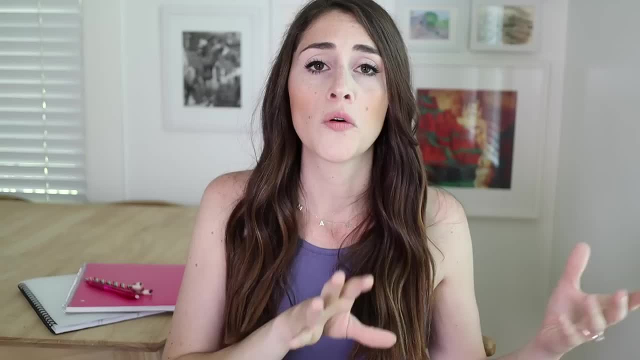 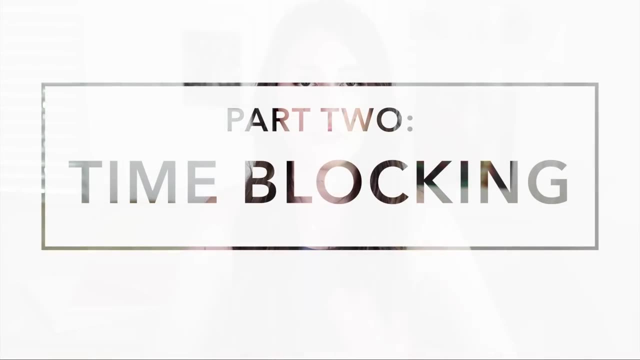 They don't get forgotten, You don't stress because you never got them done. Of course, we're trying to avoid procrastinating, but there's still that idea that there's always tomorrow too. Okay, so now it's time to move on to my second method, which is time blocking. 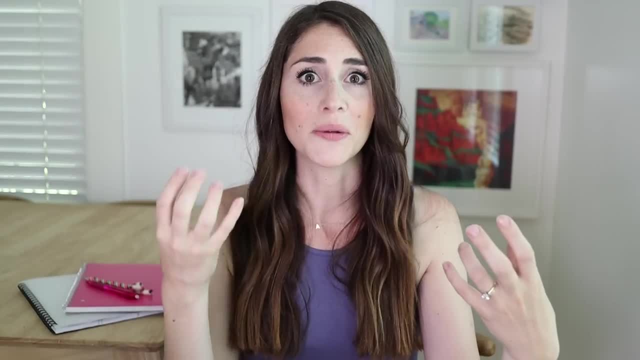 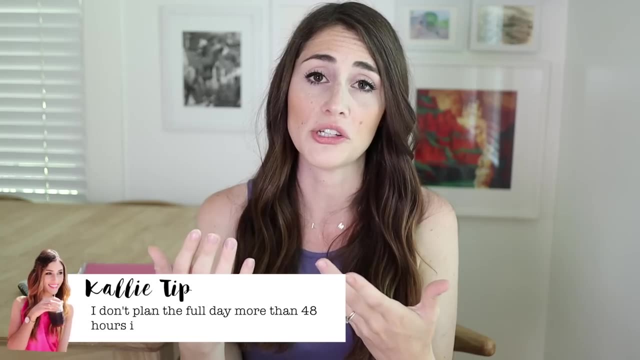 This is essentially where I take what I want to get done and I schedule in the time to do it. So once I have my monthly list and my weekly list, that's when I then schedule it out day by day. Basically, usually what I do is each morning or night I look at my day and I sort of cherry pick the tasks that I know that I'm going to get done in the next day. 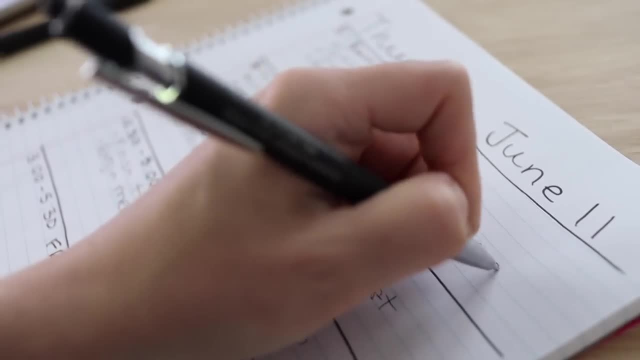 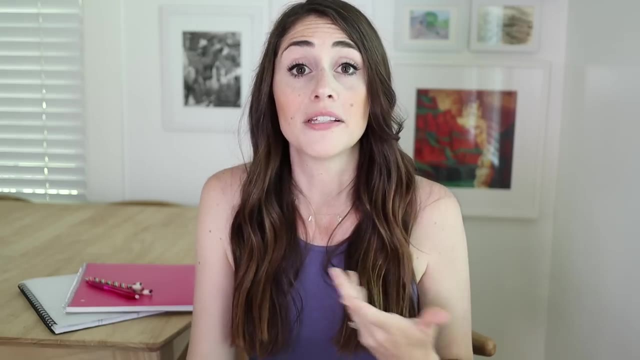 And I plan out my day using time blocking. So if you've never used time blocking, I'm going to walk you through exactly how it works. But the reason that it really works for me is because I find that our general life, especially with kids, 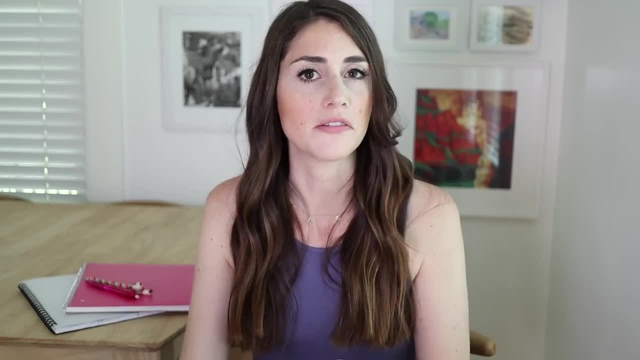 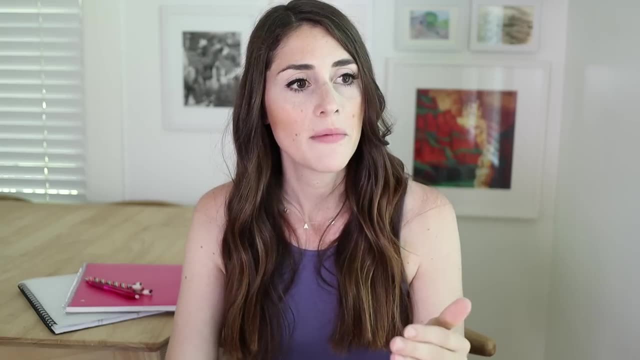 tends to just fall into this: Natural rhythms and natural blocks of time. I find that time blocking is really effective because it allows me to know exactly what I want to get done in each block of time, But it also gives me the flexibility in the breathing room that I need as a mom of a one-year-old. 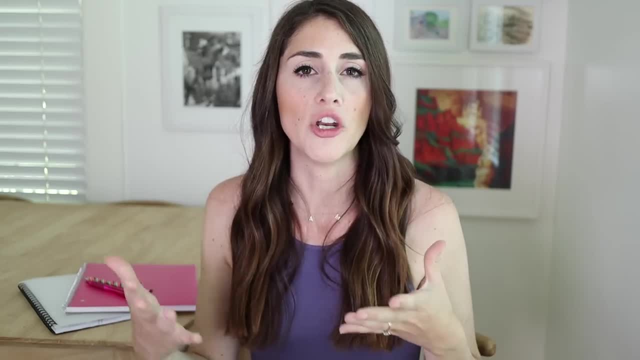 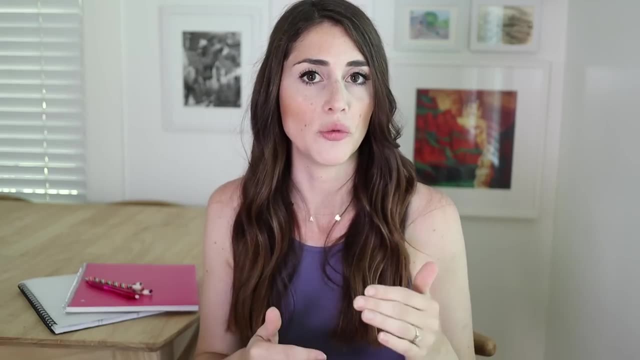 I don't feel like I'm kind of like running around like a chicken with my head cut off, not knowing exactly what project to start when, because I've really got my blocks of time planned out and I know what I'm doing in each one of them. 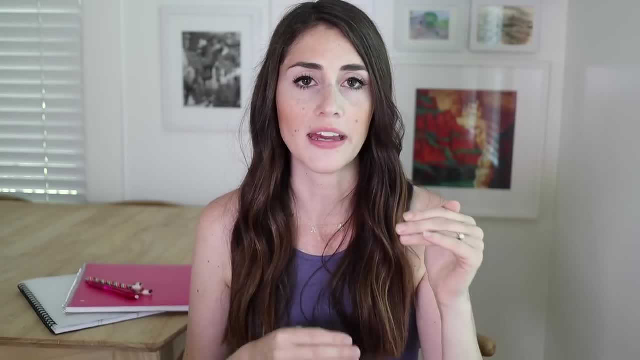 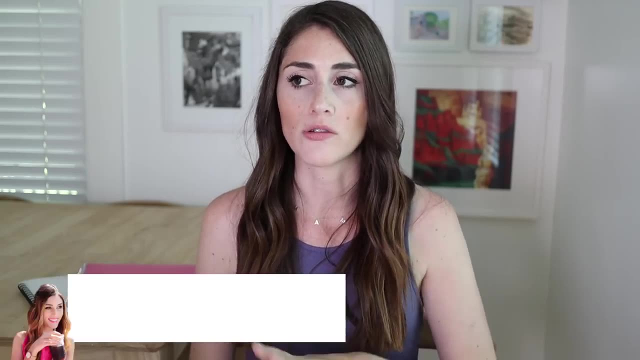 And, of course, because there's only only so many time blocks every single day to fill, I feel like it has been hugely helpful for me personally in prioritizing my list. Like I said, I was one of those people that would get really overwhelmed when I would look at my list. 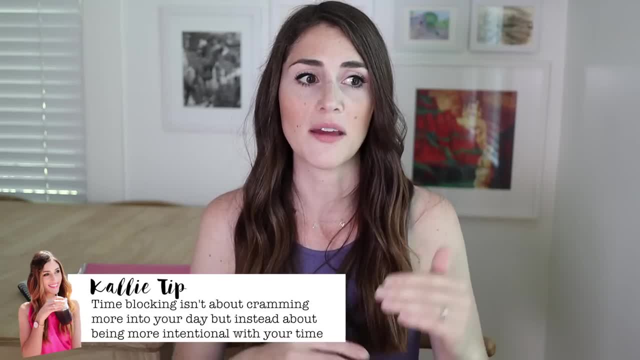 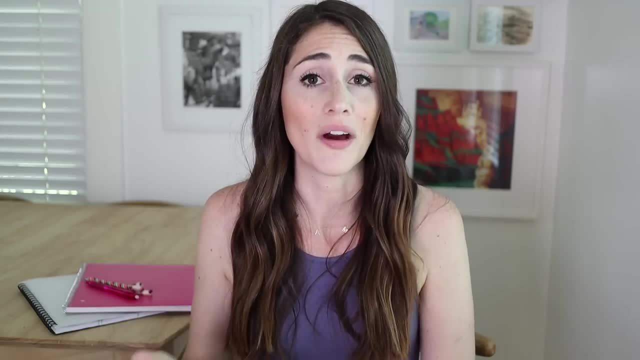 I wouldn't always know where to start And by only having so many blocks of time and each block of time dedicated to different types of tasks, it allowed me to really get good at prioritizing what it was I wanted to get done now and what things could wait until tomorrow or next week. 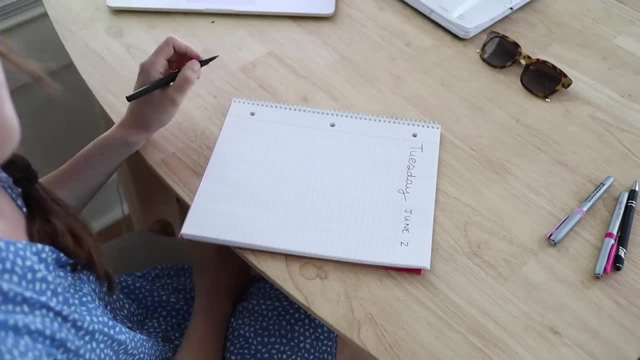 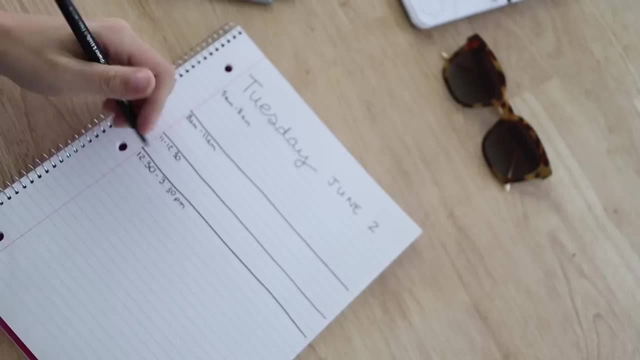 Okay, so how does time blocking actually work? and actually look, Let me walk you through it. So, using the natural rhythm that likely already exists in your day, you're going to start by dividing your day into blocks. Typically, you're looking for blocks that are like two to four hours. 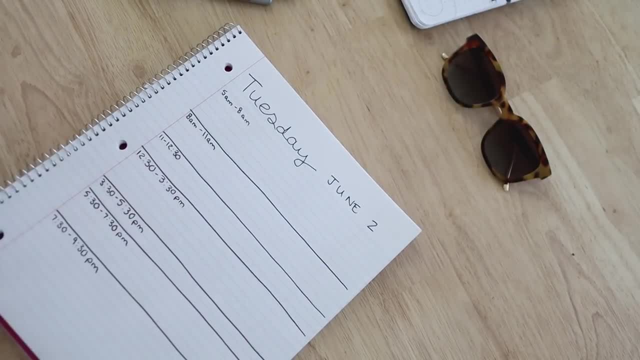 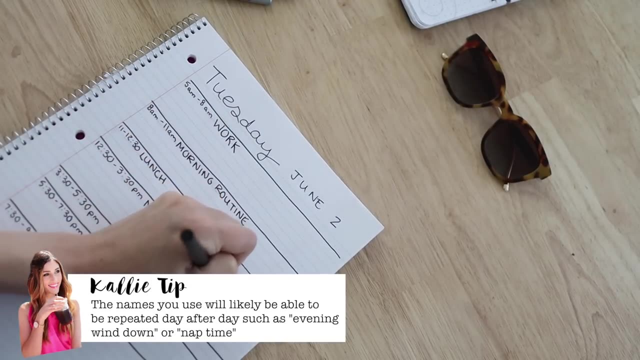 but some may be a little shorter, some may be a little bit longer. And then you're going to start by naming these blocks with generic names instead of getting specifics. So, for example, my first block, every single day before Miles wakes up, is just labeled work. 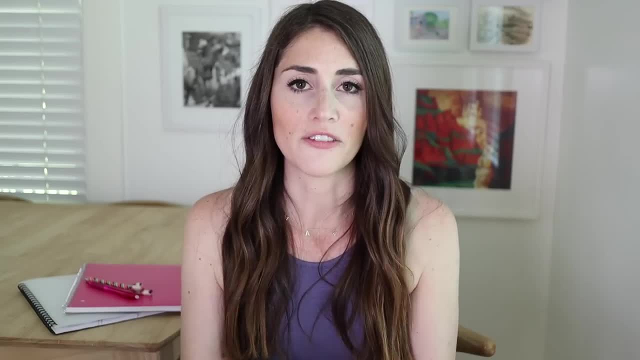 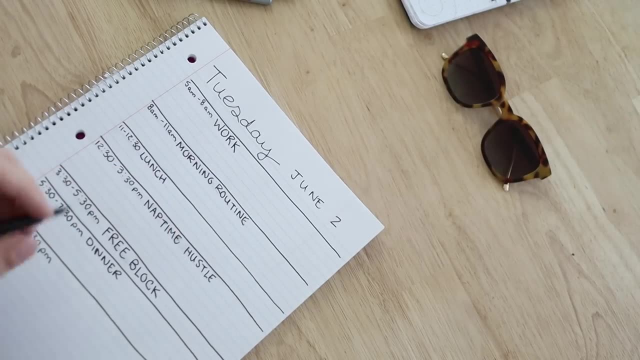 This is a work block for me. I'm going to make these a little bit more specific with specific tasks later, But for right now it's just creating generic blocks. My next block is always more specific, So I'm going to create a block called morning routine. 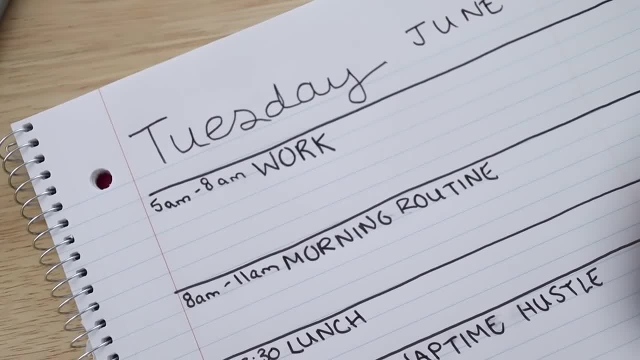 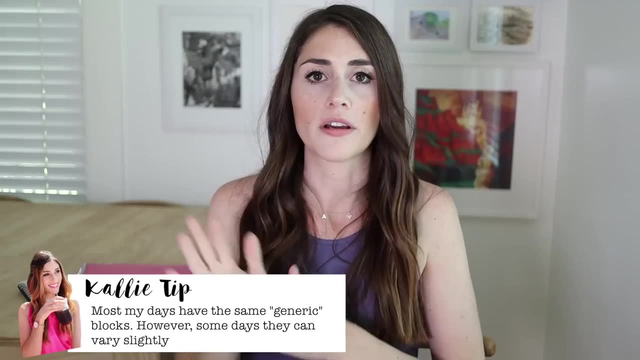 So you're just blocking out your day with general topics and working around the natural rhythm of your day. You already know, like when it's lunchtime and when do you have dinner and when does your kid nap- if your kid naps, or you know. 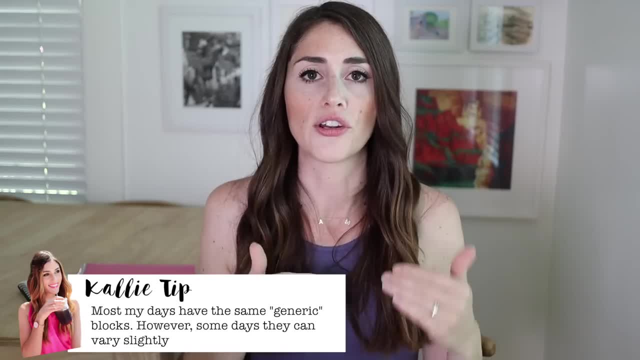 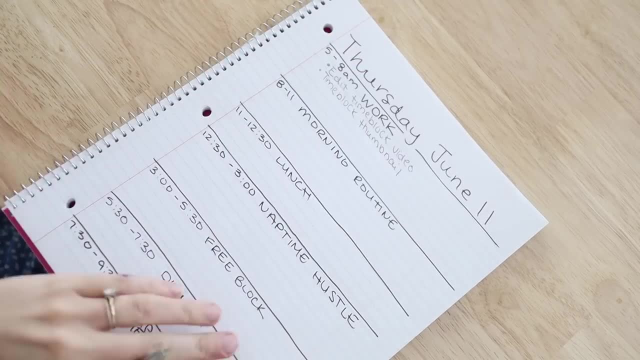 maybe your kid has a half an hour of TV time, always at 2 o'clock. You already have some natural rhythms. You're going to create your blocks around that, Okay. so once you have your general blocks, this is where you start to add in your smaller tasks. 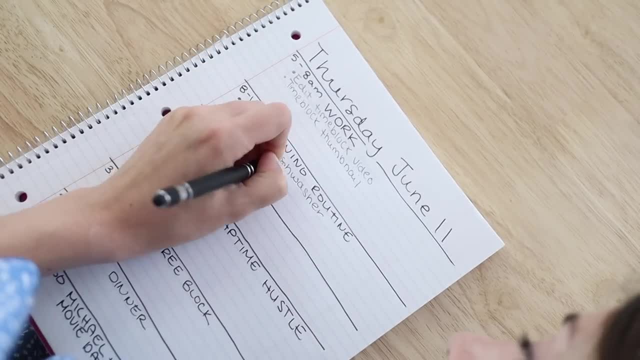 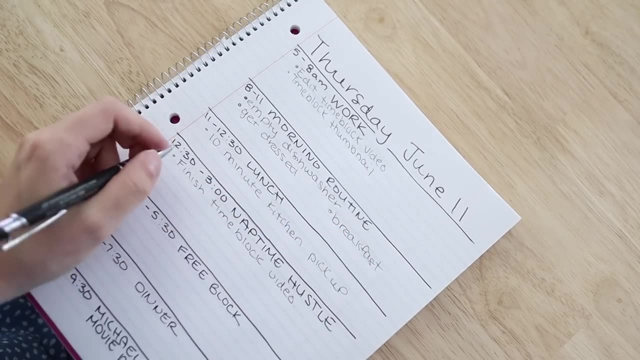 You want to write down everything you want to accomplish in that block. So I'm going to create this block called morning routine and inside of that block every day is: have breakfast, empty the dishwasher, get me dressed, get Miles dressed. It's not to say like 8 o'clock, we have breakfast 8.30, we get dressed, 8.45, we empty the dishwasher. 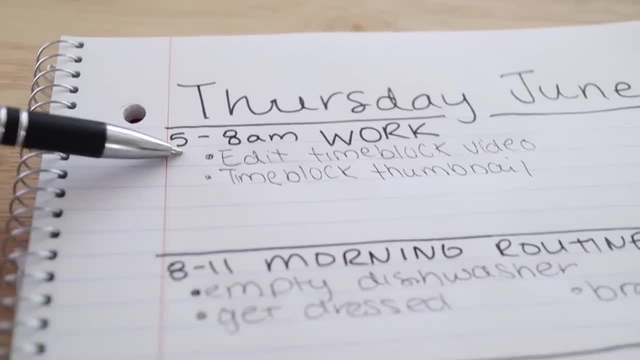 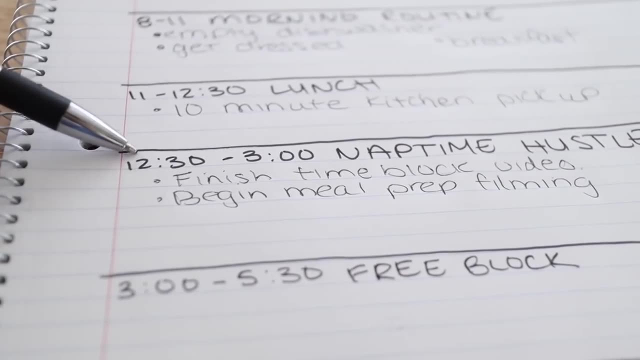 It's just that between 7.30 and 9.30, these are the handful of things that we need to get done, And then you want to be blocking similar things like tasks together. So for me, my first block of every morning, like I said, is a work block. 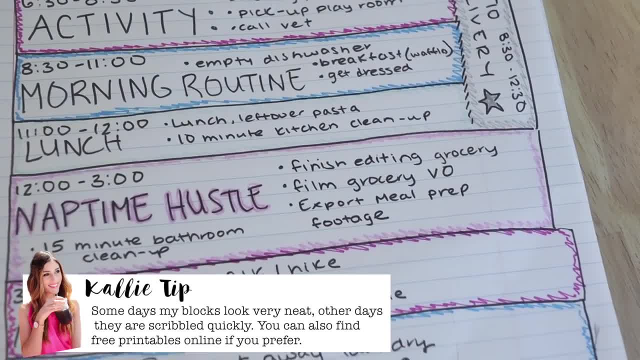 So this is what I'm going to be doing: work tasks. I'm responding to emails, I'm editing a video, I'm writing a blog post. I'm doing all tasks that pretty much require me to be sitting down at my laptop. 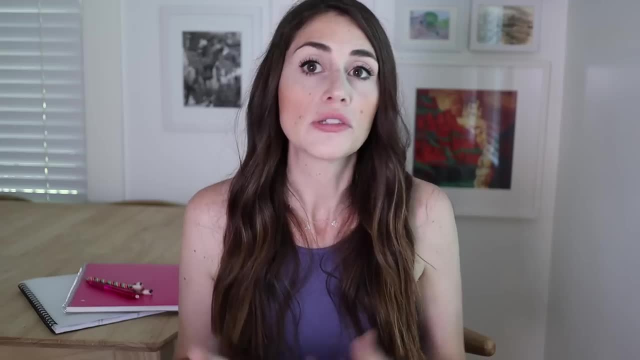 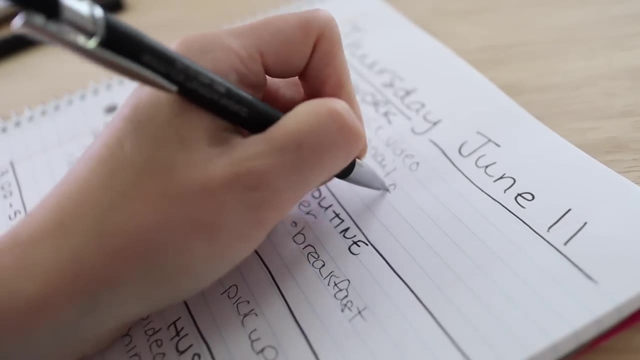 The next two blocks of my day are more like home personal blocks. This is when I would get things done like laundry or, you know, like dusting the top of the cabinets or whatever. The basic idea I'm trying to say is: you want to block together similar tasks. 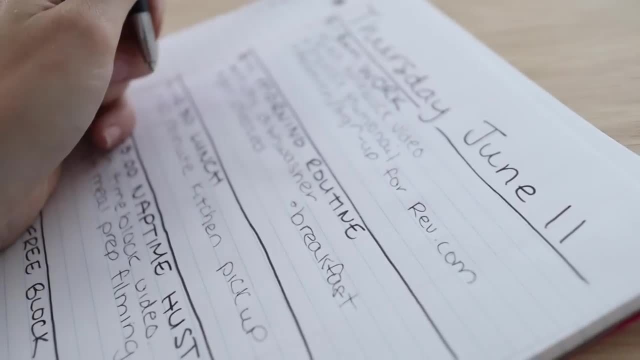 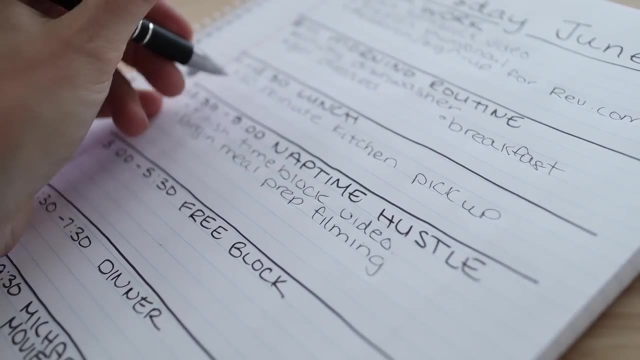 because you don't want your brain to be switching between all of the millions of tabs. So if you have a three-hour block and you have a handful of things in one category and a handful of things in another category, split that into two. 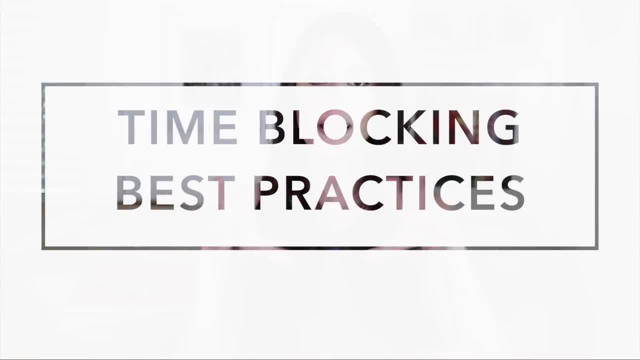 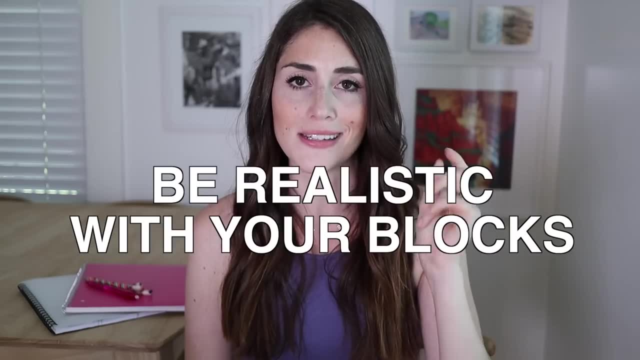 Okay, so now that you kind of know how time blocking works, I have a few very important like tips to make it successful. Now, the first tip is to be realistic with your blocks. I think sometimes we will see a block of time that's two hours. and think that we can do 20 tasks, but it's honestly not realistic. Remember that most tasks take longer than we think. Plus, life happens. We get distracted. our toddler spills our milk, somebody gives us a phone call and we get caught up doing that. 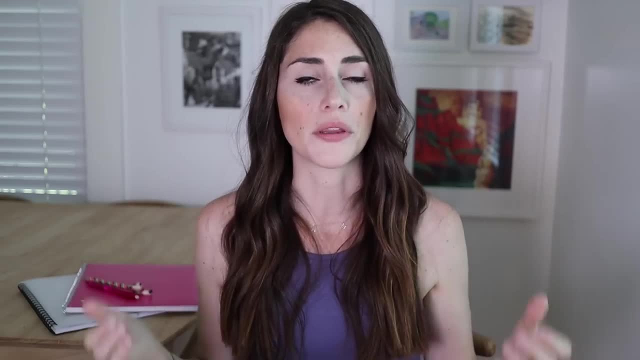 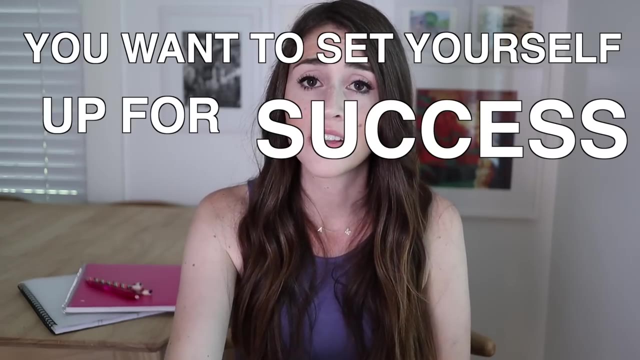 Life is going to happen and you need to give yourself that flexibility in the breathing room to allow that to happen. It's the reason that block scheduling works. The point is, you want to set yourself up for success so that at the end of the day, you feel accomplished and not defeated. 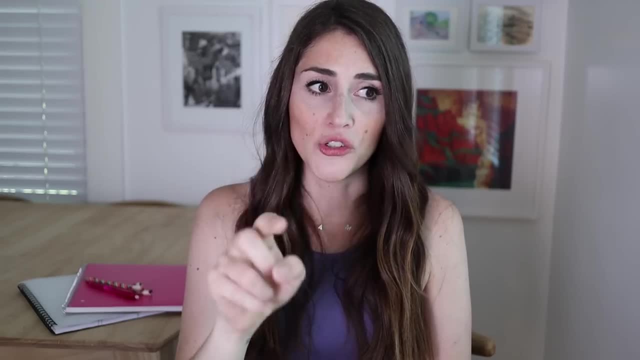 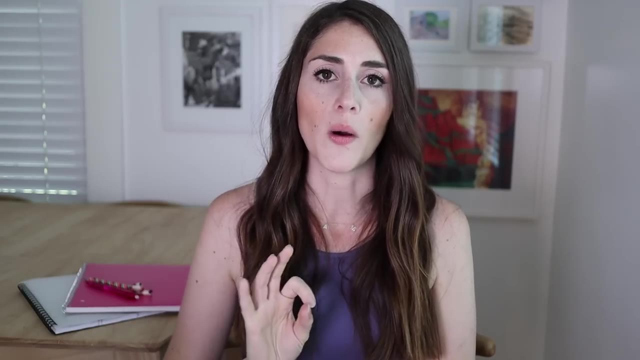 This is important and this one's on you: to make sure that you're doing it right. Don't overextend yourself. Be realistic with your time blocks and what you can get done in each one. Tip number two: especially helpful if you are a mom in it. 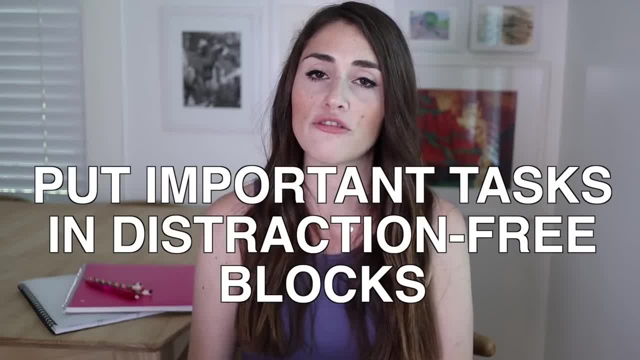 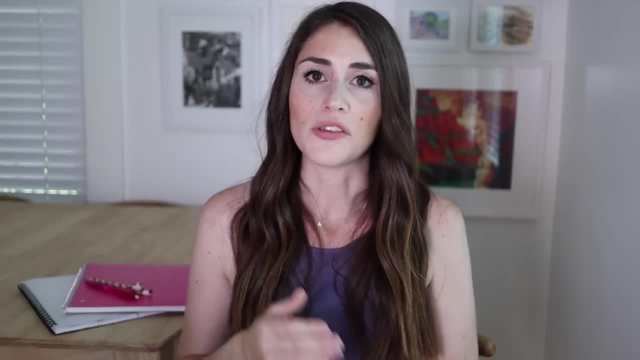 while you're trying to do this is to put your most important tasks in distraction-free blocks. So for me, all of my work-related stuff needs to happen, usually when my son is not around, So these are morning blocks before he wakes up. 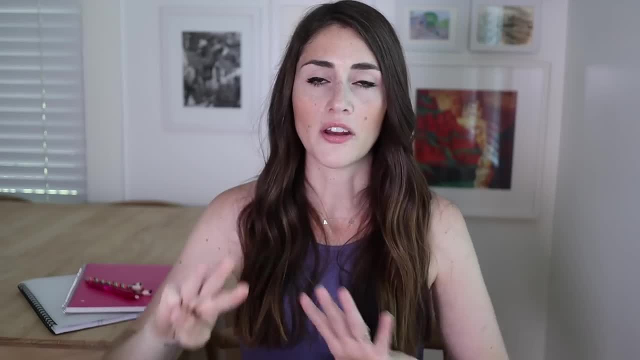 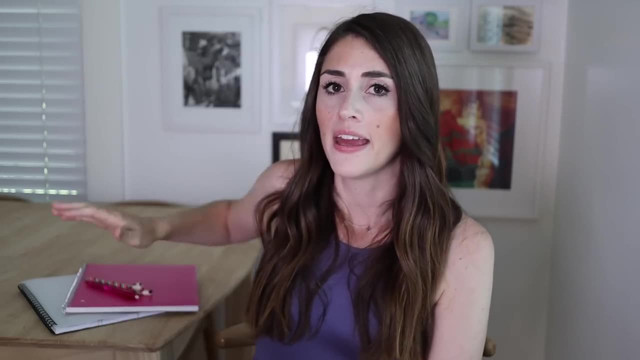 nap time blocks or blocks after he's gone to bed? Okay, third tip and a question that people will probably are sort of wondering is like where to do this. Obviously, I've been showing you my schedule. I do all mine in these two notebooks. 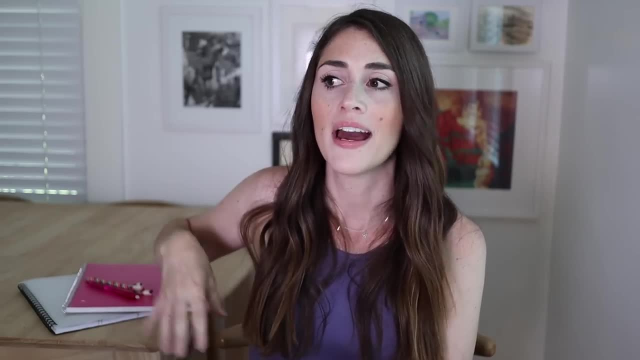 So I use pen and paper, and what I like about this is it's portable, So I literally can be sitting on the sofa, I can be writing down my schedule or my- like- monthly list for that month And I can sort of take it with me. 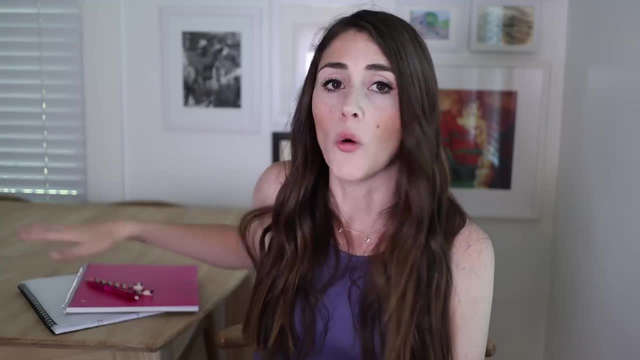 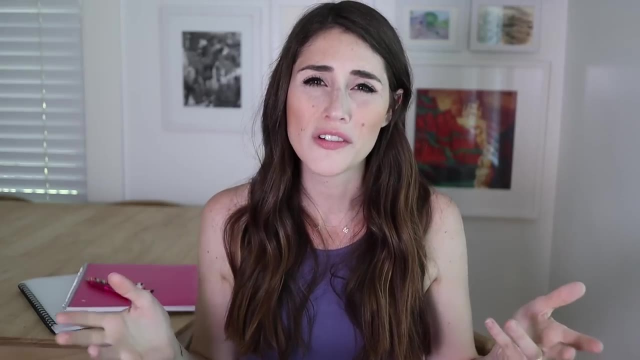 And then usually throughout the day, this notebook sits open on this table, which is essentially like in our great room, So it's always at a quick place where I can see it. I can always reference it. You could go for something hanging on the wall like a weekly whiteboard calendar. 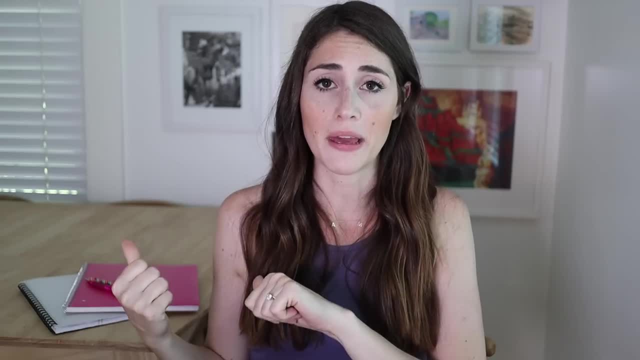 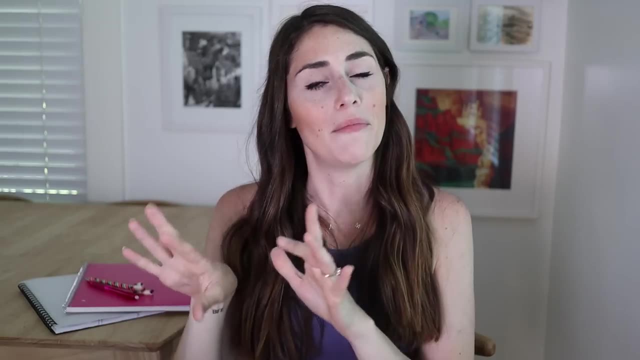 But personally I don't find that quite as effective. I find the pen and paper to work really, really well, like I said, because it's portable and I can take it around with me. Another note is I do not like to do any of my scheduling on my phone. 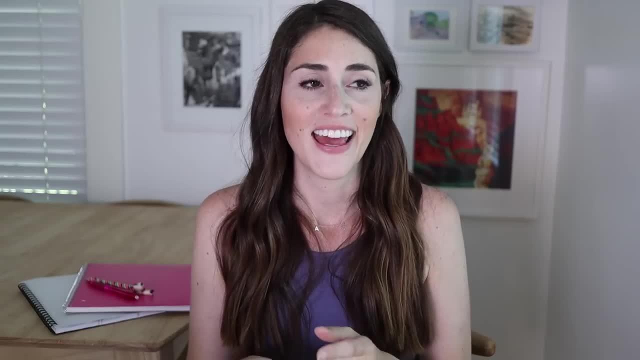 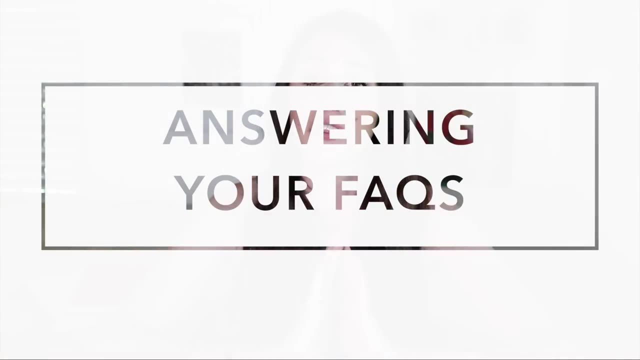 I don't use apps for this because phones are extremely distracting And I don't want to open up my phone to see what I need to do and then get distracted by notifications or something else along those lines. Okay, the last thing I want to do is jump into a bunch of FAQs. 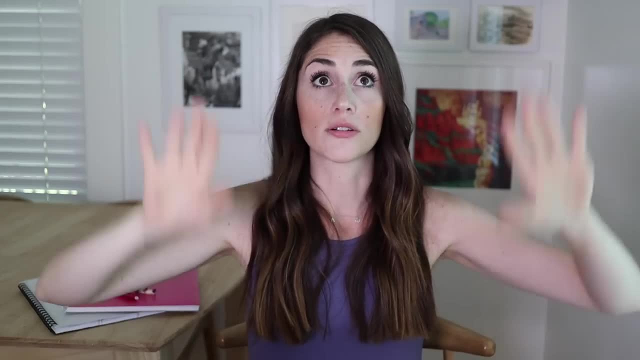 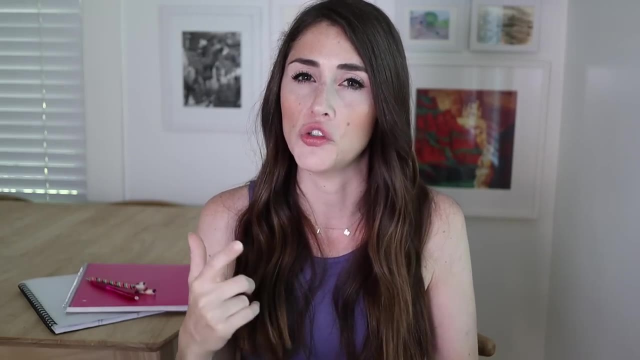 that I got directly from you guys. I'm going to write them all down, because there were a lot of them, into an entire blog post, But I want to touch on the most common ones that I got in this video, since it may be questions that you still might be wondering when you're like. 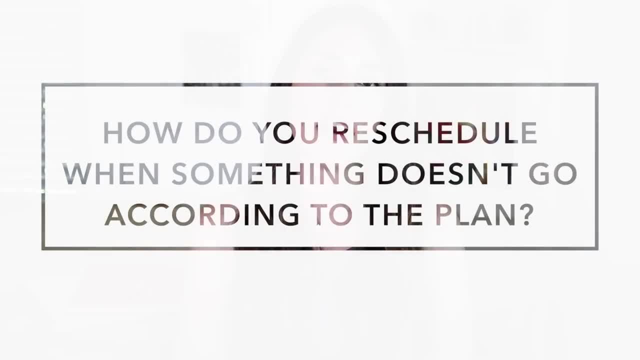 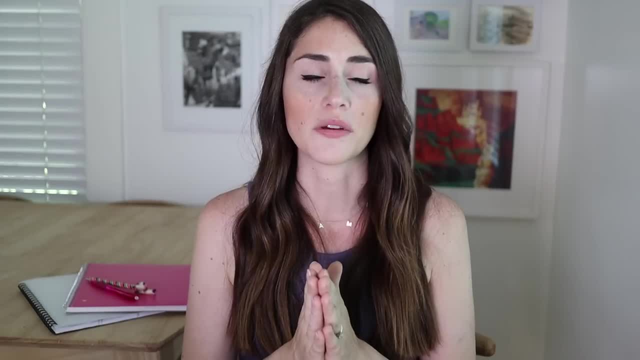 okay, how do I make this happen? Okay, first question is: what do you do and how do you reschedule when something doesn't go according to the plan, Essentially when the day goes off schedule? So, in my opinion, the best method here and the reason that time blocking works: 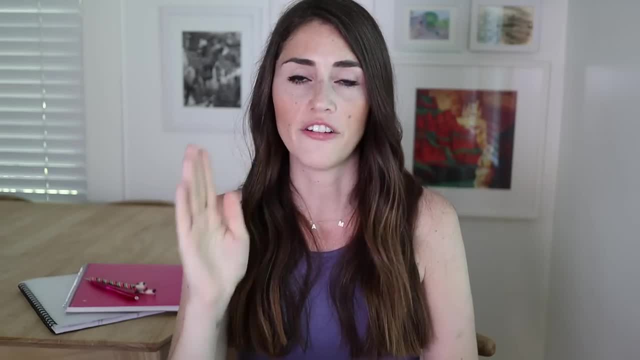 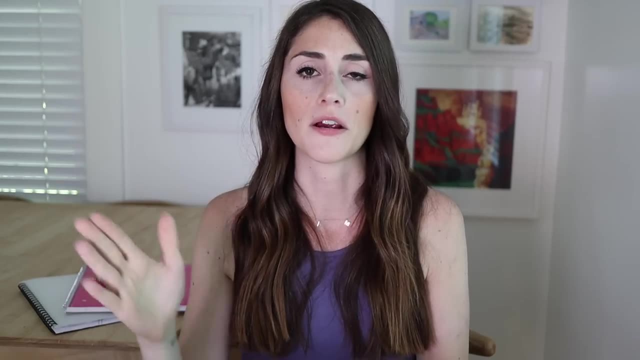 really well is just say like okay, this block is a wash, start fresh on the next block. Or if it's like a really big something that happened, start fresh tomorrow. Whatever you need to do is start fresh two blocks from here. 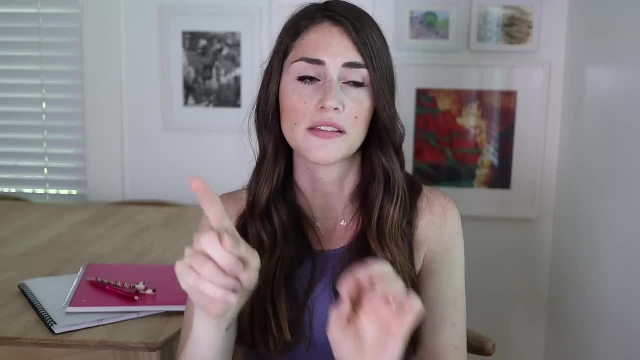 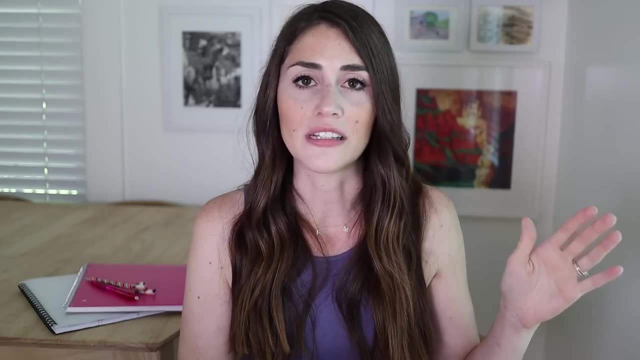 Life happens and it's going to happen and we don't want to get stressed about it, And this is the reason. also, having the master running list is really great, because whatever was supposed to happen in those blocks, you still have them over on your master list. 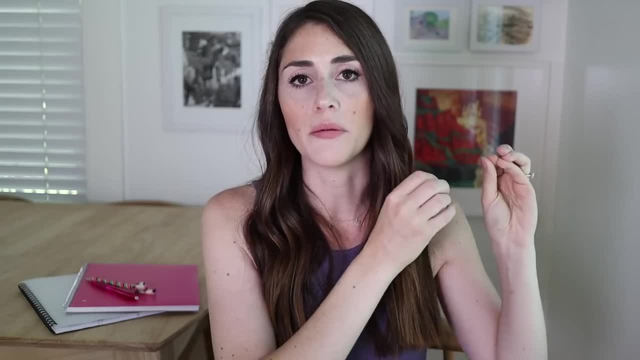 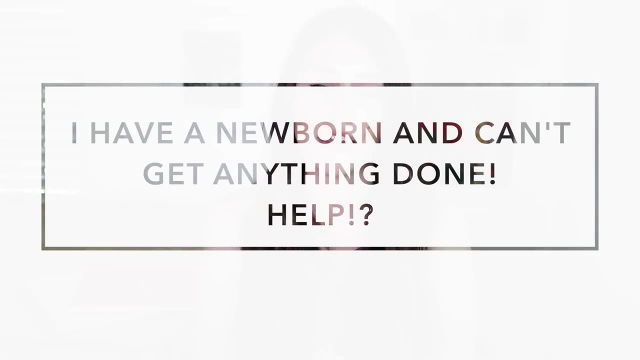 And when you make tomorrow's time block or the next day's time block, you'll be able to make sure you still get those things done, Okay, so the next question said: my baby is two months old and always needs to be on me and I literally cannot get anything done. 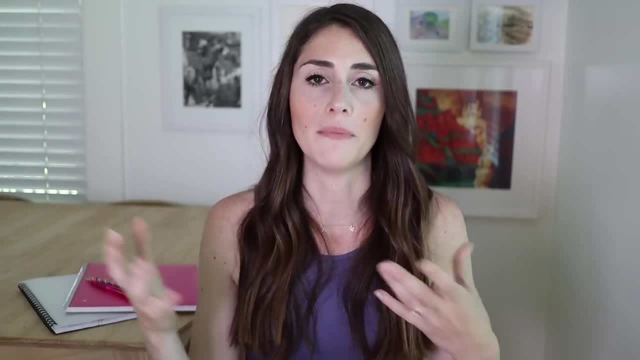 And I got this version of this question from like a million different moms who are, like you know, I have a newborn. My kid is six months old. like I can't get anything done, I'm always watching this kid. like how do I do it? 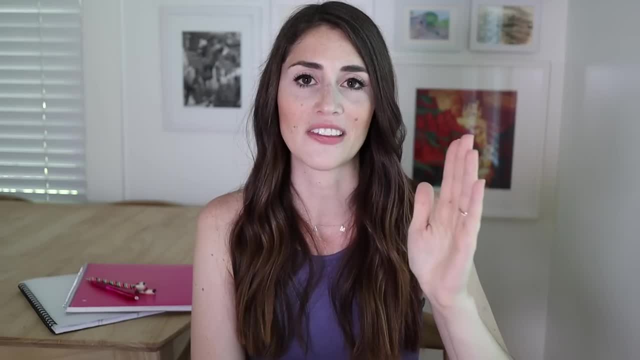 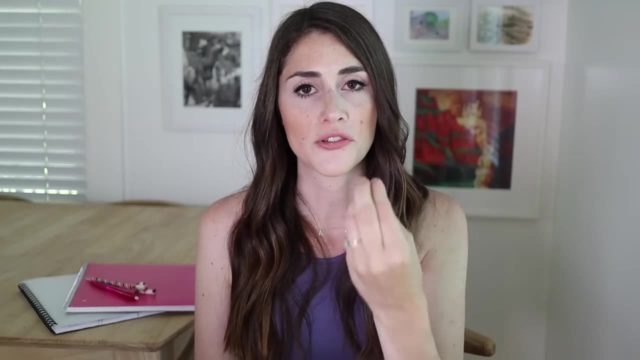 I told you guys my sort of productivity journey at the beginning of this video. So I totally get it And I was there. motherhood kicked my productivity in the butt. So let me just promise you that your schedule will return. I know things feel a little bit upside down right now. 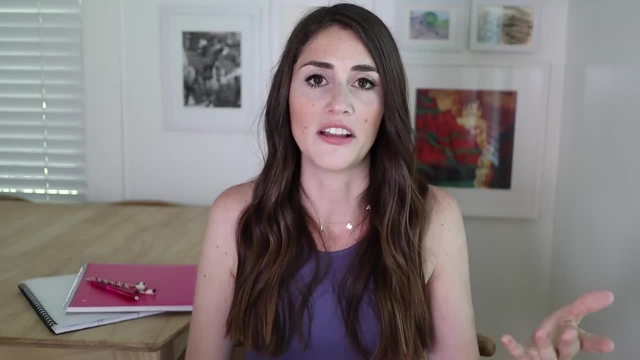 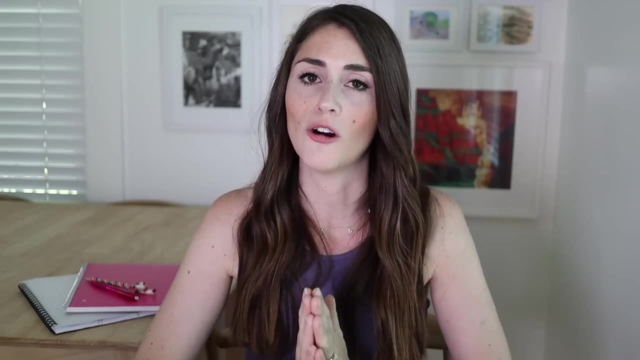 but your schedule will return. that being said, I also understand that you sometimes still like want to get some stuff done. You're like Callie, That's fine. I love my newborn be like and please need to have clean laundry. So I have a couple little steps that hopefully will help. the first one sounds: 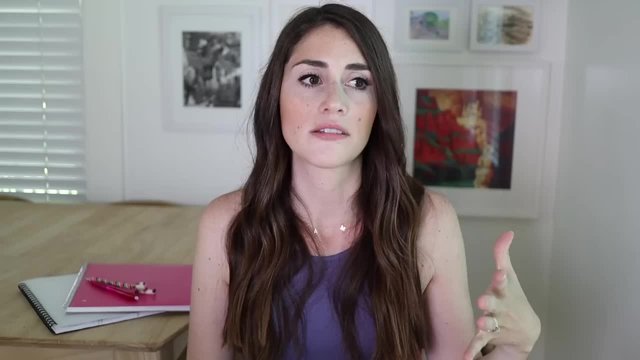 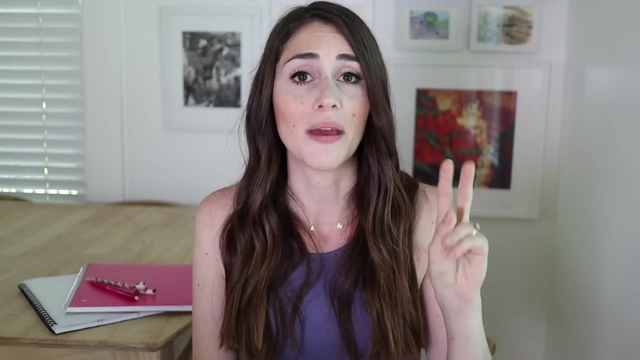 a little funny, but I'm not being funny at all, And that is just lower your standards. You can't get as much done as you used to, or maybe even as you thought that you would be able to honestly pick one or maybe two tasks a day that you want to get. 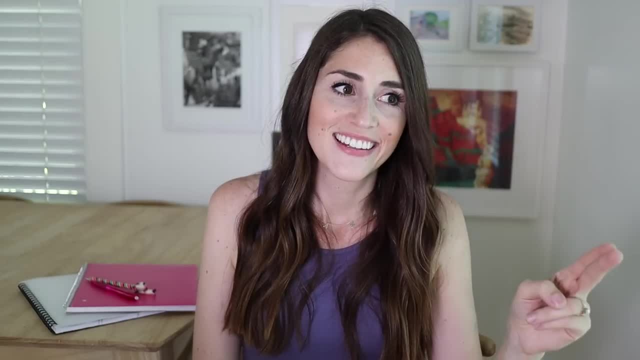 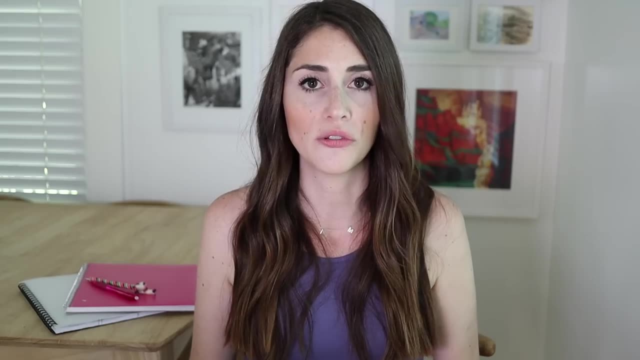 done that day Again. like I said before, it's about being realistic so that you don't feel defeated at the day end of the day. instead, you feel accomplished. So you say, like the one thing that you're going to do today is those two loads of 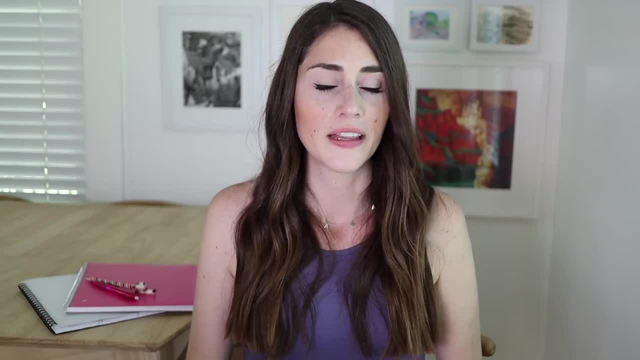 laundry and you're going to get them cleaned and you're going to get them put away. That's what you're doing today to, if you don't already use baby wearing. baby wearing is like game-changing. It's the only way I ever got anything done. 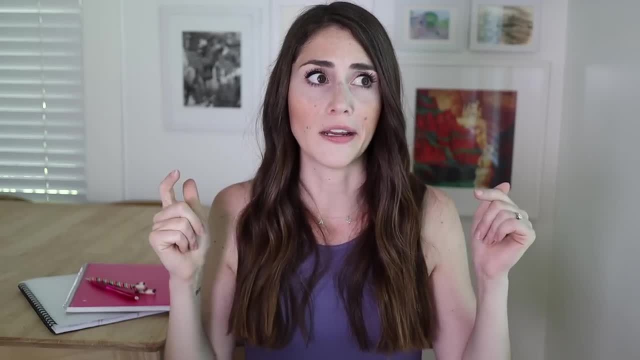 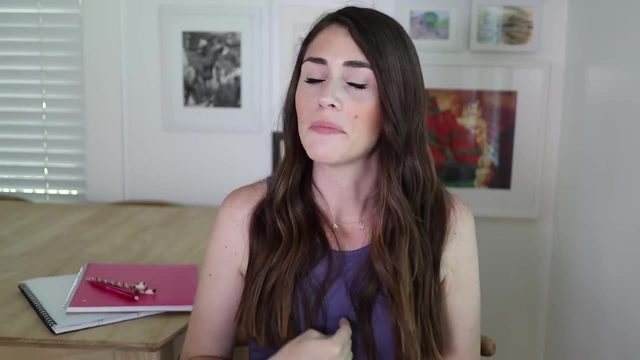 So if you're not using that already, I will link my two favorite baby wearing baby carriers, my two favorite baby carriers down below. and my third tip is: ask for help, and know this seems really cliche, but personally I am the worst person in the entire world asking. for help and I've been getting a lot better, but I still struggle with it. One thing that helped me a lot in the newborn phase is when my husband and I decided that two or three nights a week when he got out of work he would take our newborn son and 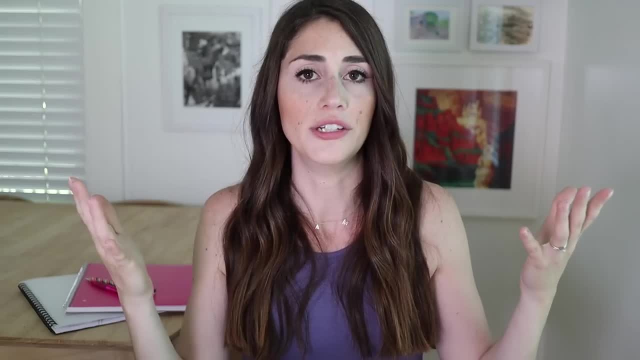 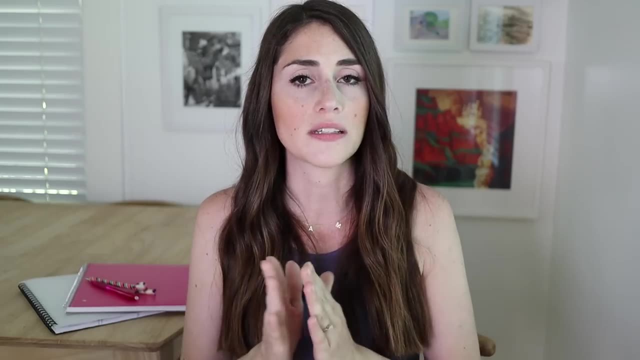 I would have like an hour or two hours for whatever I wanted to do, whether it was work, shower, take a nap, do the laundry, like whatever it was that I wanted to do. and it was a sacrifice because I was losing a couple nights a week. That was family time, but it was necessary to happen. 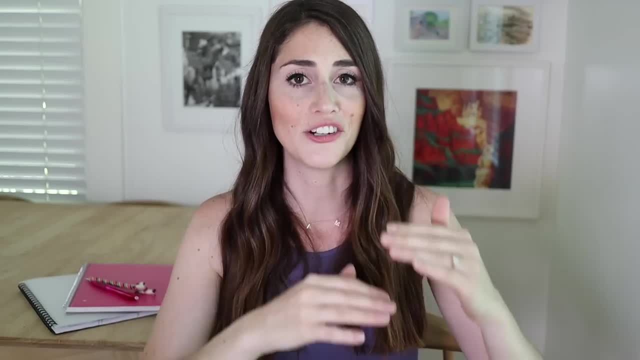 What's really important is you want to schedule those days in. they need to be in your time blocks, It's not? you just tell your husband like hey, a couple nights a week Will you take the kid? It's like you're like what is it? Thursday and Tuesday? 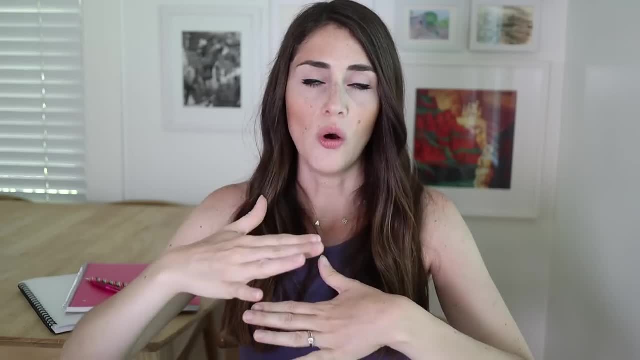 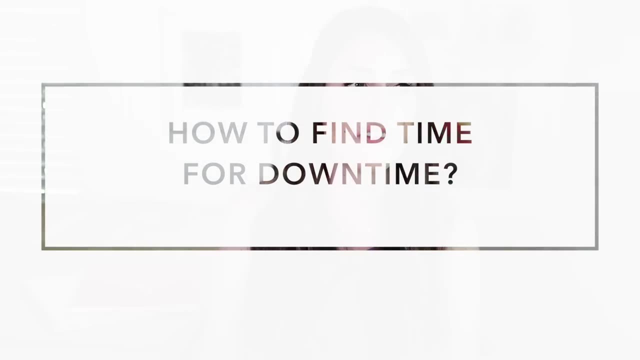 Okay, great, I'm writing it into the schedule and then you know you have those blocks of time and you can fill them with tasks that you're going to get done. Another very common question is: how do you find downtime, How do you find time for yourself, time to relax, and, honestly, you block it in. you find 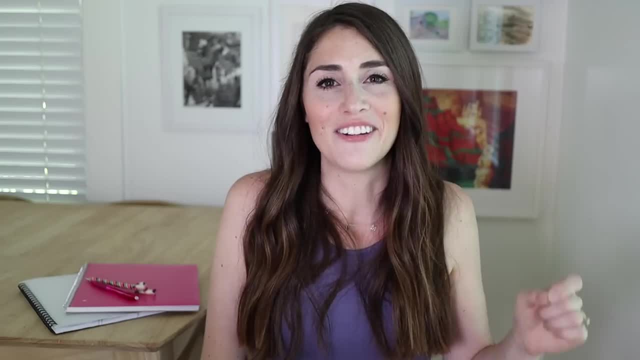 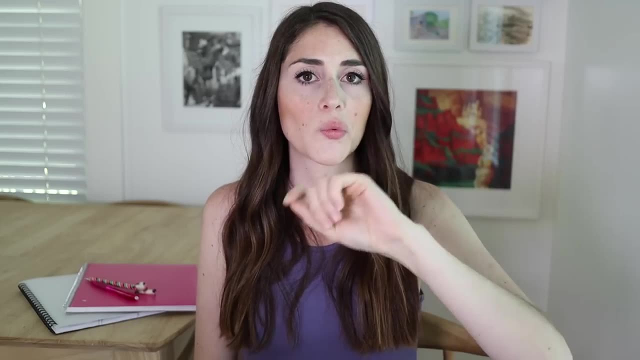 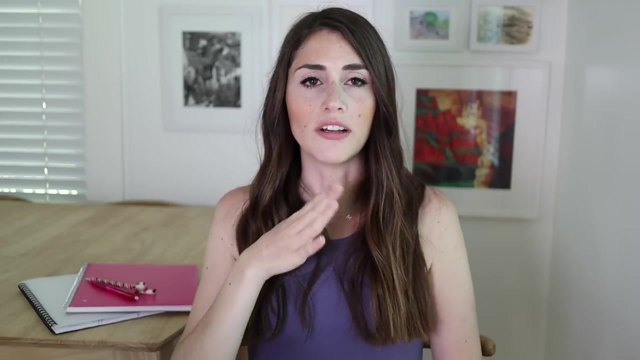 a time Block seems sort of silly. You're going to write like relax down into a time block, but that's literally what I do. I will literally write a block of time that says family time or like relaxation, or like do nothing whatever. I block it into my days and I know that the idea of like blocking 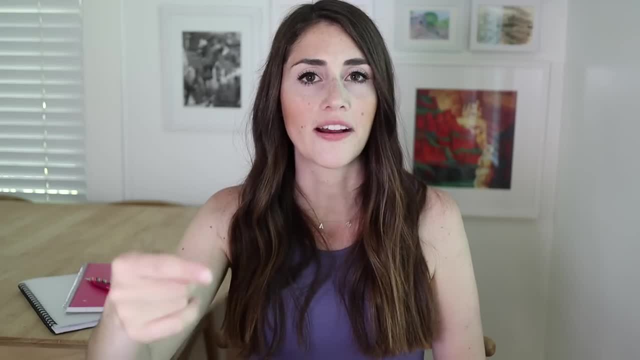 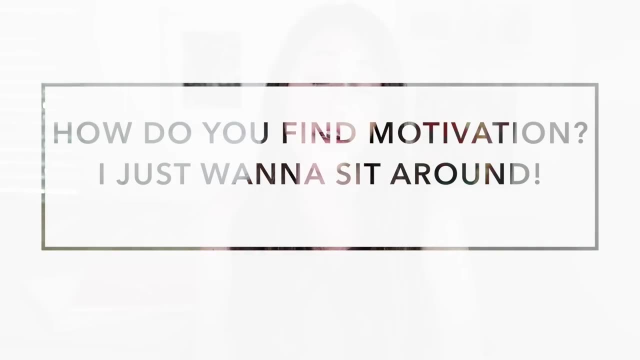 in downtime seems a little bit over scheduled, but it actually ends up being the opposite and it actually leads to a schedule That's like far more relaxed. Next question is: how the heck do I get anything done when all I want to do is sit around all? 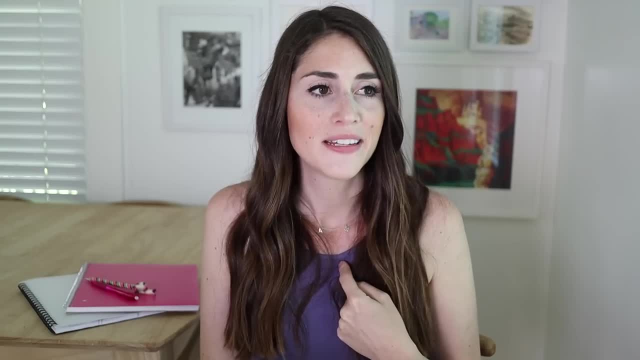 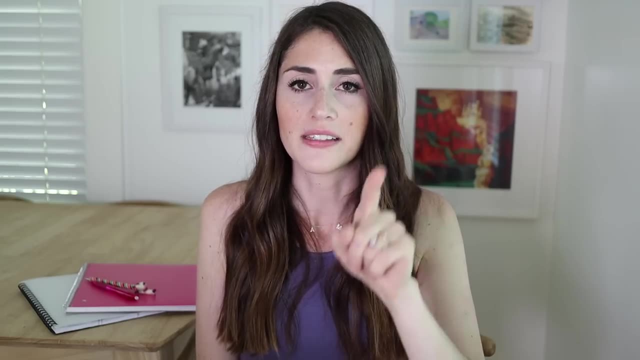 the time I get it. Don't think that I have not been bit by the just want to sit around all the time bug, because I totally have. but I've learned one very important lesson, and that is that a body in motion stays in motion. 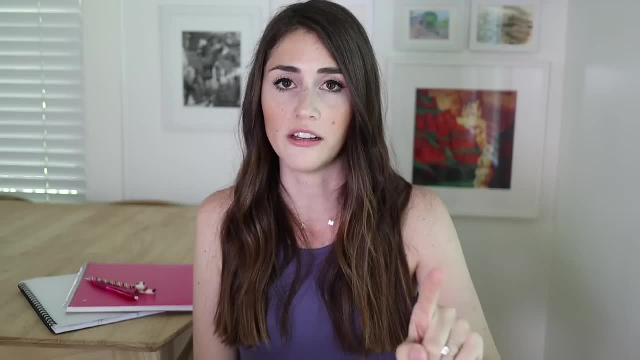 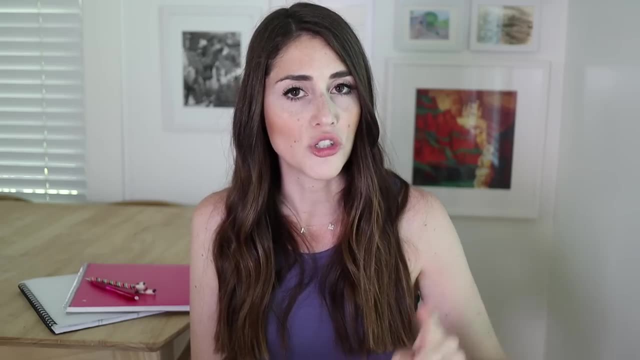 So when I'm sitting around and I'm feeling lazy and I don't want to get up, I force myself to get up and do one task. say, okay, I'm going to get up and do this one thing, and I find that usually 90% or more of the time that doing that one tasks gives. 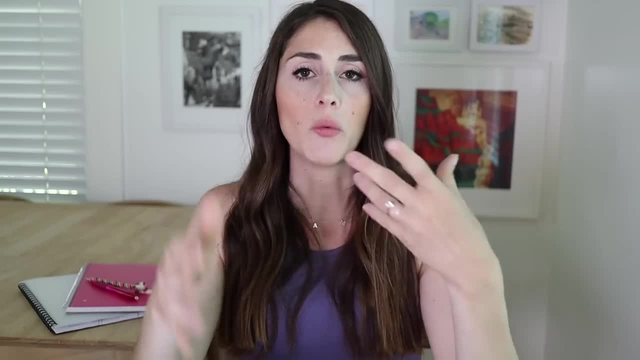 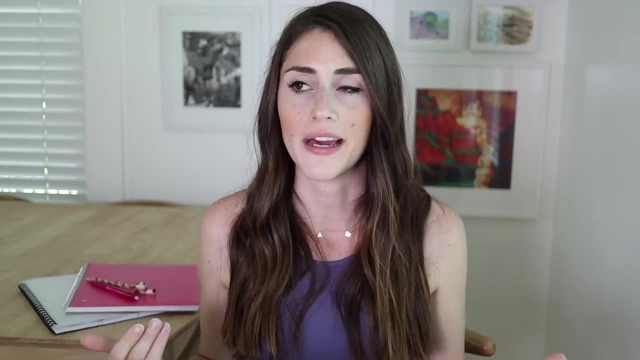 me a little bit of momentum and it gets me moving and it gets me wanting to do the rest of the task. And for the other 10% of the time, Oh well, your body needed a break. It's telling you you need to sit down. take the task from that time block and put them. 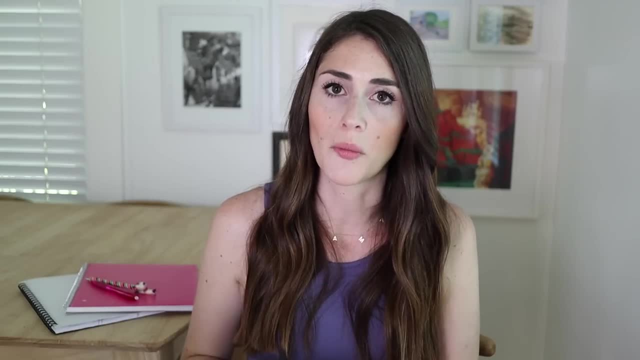 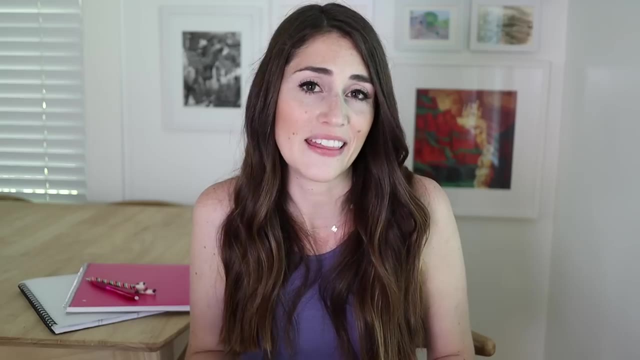 in tomorrow. Okay, Like I said, there's a lot more FAQ, some of them a little bit more specific, So I'm going to answer all of them in a big, huge blog post. some of the other questions that I answer include things like: how do you get anything done if your baby won't take?